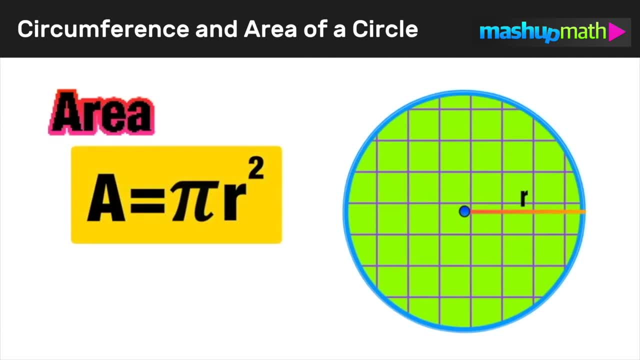 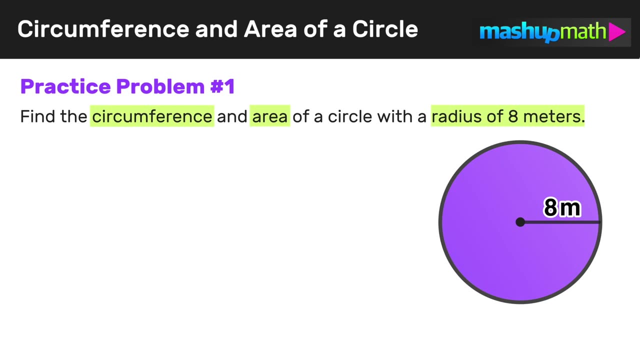 at a few practice problems on how to apply these formulas to find both the circumference and area of a circle. Okay, so here is our first practice problem. We have to find the circumference and area of a circle with a radius of 8 meters. 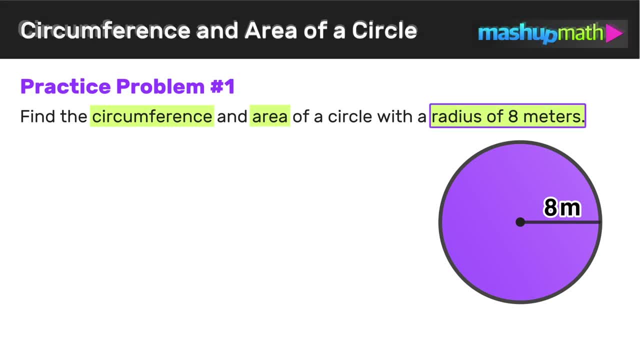 So correctly identifying the radius of a circle is key to finding the circumference in the area. So in this example we know that r is equal to 2 pi r squared. That is given to us And now we can use the circumference and area formulas. 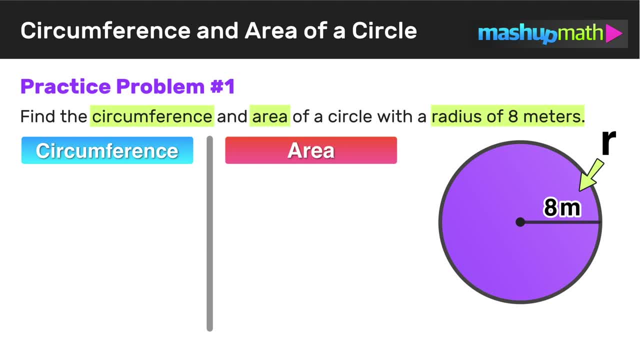 to solve this problem, since we know what r is. So let's start off with circumference. The formula for finding the circumference of a circle is c equals 2 pi r. So in this case we have c equals 2 times pi, times 8,, since we are replacing the radius with a circle. 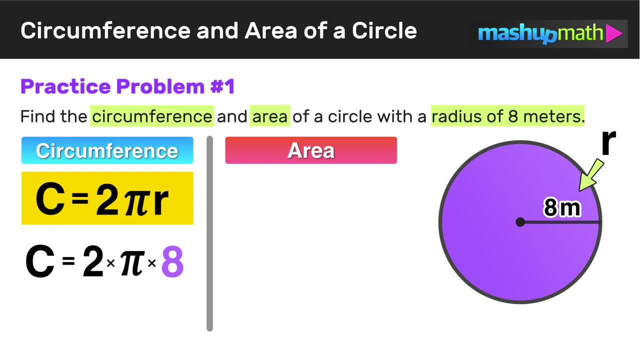 Now all we have to do is multiply, And we can actually use the commutative property of multiplication here to rearrange the terms. So let's rewrite this as 2 times 8 times pi, And doing this lets us express our answer in terms of pi, since we know that 2. 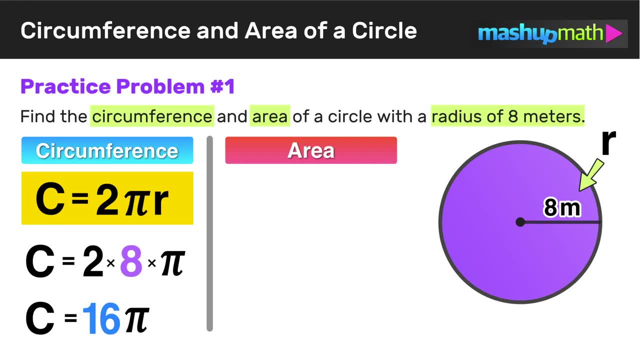 times 8 is equal to 16.. So if you wanted your answer in terms of pi- some questions will ask you for that- the circumference equals 16 pi. But if you wanted an exact answer, you have to take one further step and multiply 16 by pi and we will get an. 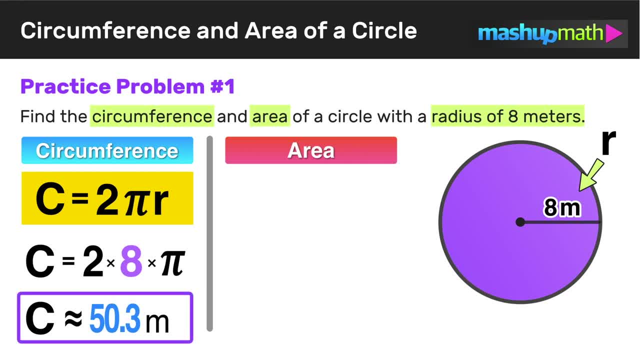 approximate answer of 50.3 meters. So for this example, the circumference of the circle is approximately 50.3 meters. So now let's go ahead and find the area. So now we're going to use the area of a circle. formula a equals pi r squared, And again we have: 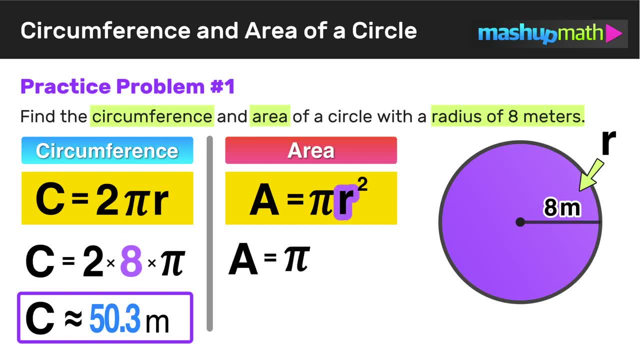 to substitute r, the radius value, with 8 for this example. So now we have a equals pi times 8 squared. and now we just have to solve. So we know that 8 squared is equal to 64, so we have a equals pi times 64.. So again, if you wanted the answer in terms of pi, the area would: 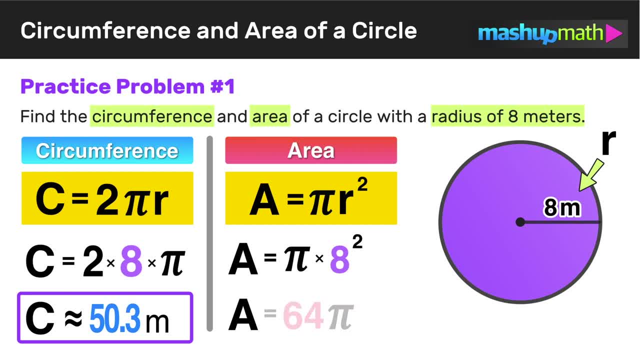 just equal 64 pi or 64 times pi, but if you wanted an exact answer, you just have to multiply. 64 times pi is approximately 201.1 meters squared, and remember that area is always represented in square units. Okay, so now that you have some experience with using those circumference and area of a circle, 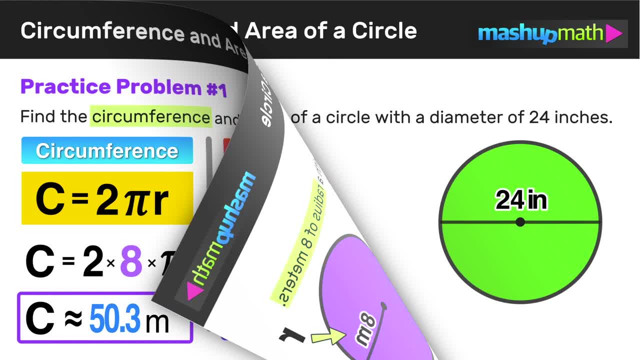 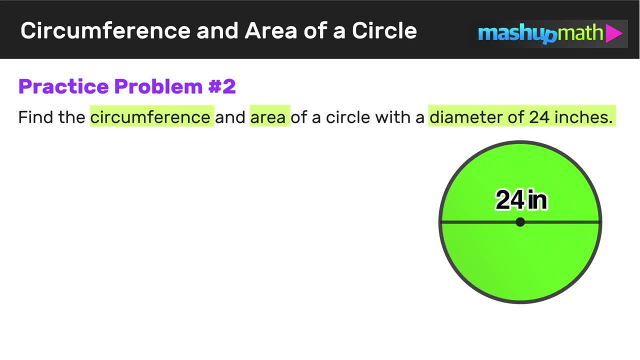 formulas. let's go ahead and take a look at another example. Okay, so here's practice problem number two: And we have to find the circumference and area of a circle with a diameter of 24 inches. So this example is a little bit different, because we aren't given the radius, we're given the diameter. 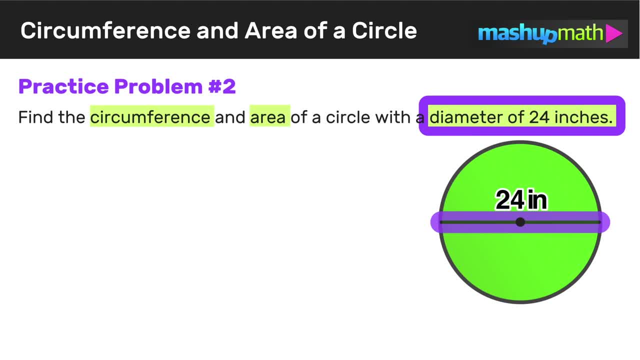 But we should know that a radius is equal to half of the diameter. So if the diameter of this circle is 24, we have to ask ourselves what number is half of 24, and we should know that that number is 12.. So, because we know the 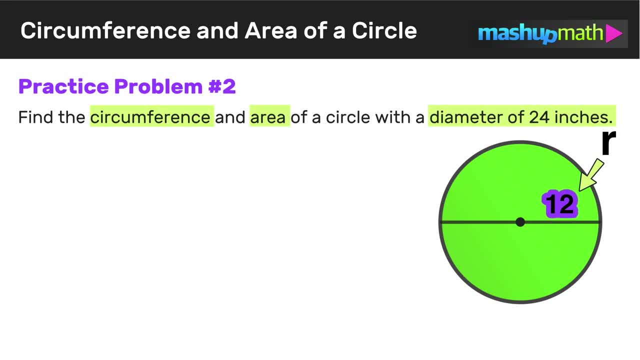 diameter of this circle is 24,. we also know that the radius r is equal to 12.. And now that we know the value of r, we are ready to use our formulas to find the circumference and area of this circle. Starting with circumference, we'll use the formula: c equals 2 pi r, so in this case, c. 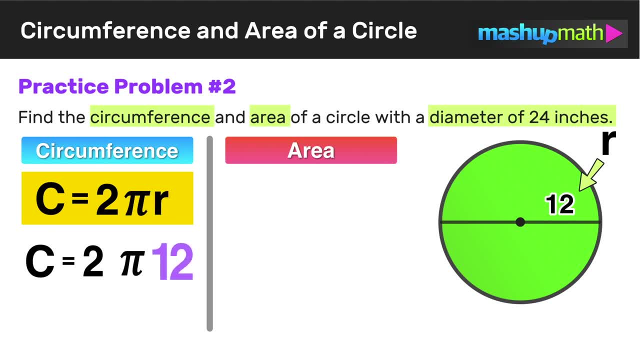 equals 2 times pi, times the value of the radius, which is 12.. And, just like the last example, we can use the commutative property to rearrange the terms. so let's rewrite this as 2 times 12 times pi. 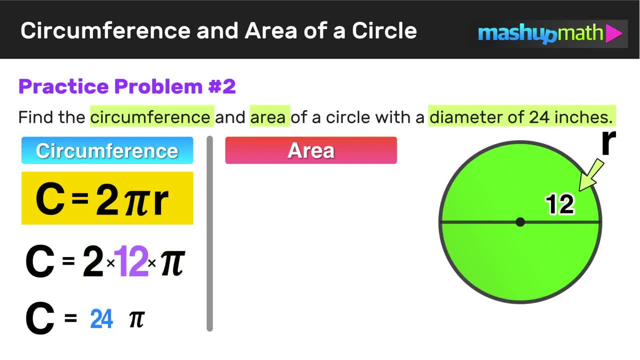 Doing this lets us easily multiply 2 times 12, which we know equals 24.. So we can leave our answer in terms of pi if we want to. circumference of the circle equals 24 pi. Or if you want an exact answer, you can multiply 24 times pi and conclude that the circumference 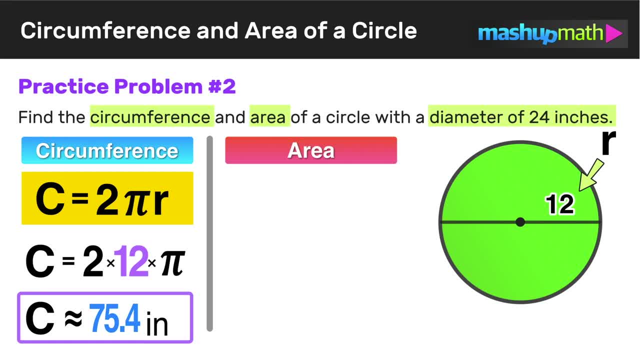 is approximately 75.4 inches. Now that we've found the circumference, let's go on and find the area of the circle. So the area formula of a circle is a equals pi r squared. So we have a equals pi times the value of the radius, in this case 12..